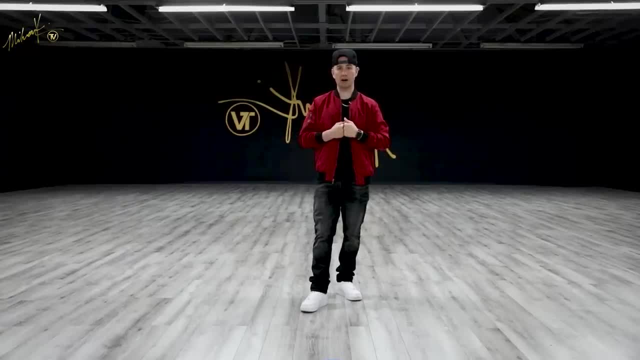 like a robot for this, And let's get into it all right. The first step is we're going to be here straight shoulder width apart with our legs, bam, okay. What I'm going to do is I'm going to twist my wrist. okay, It looks like this: 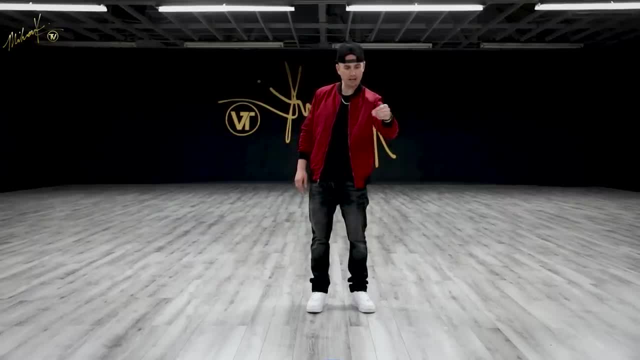 Kind of like a circle, Almost, like I'm holding a teacup, okay, Like this. So my hand's normal and I'm going to go twist, all right. So we go whoop, all right, And then we're going to bring our arm. 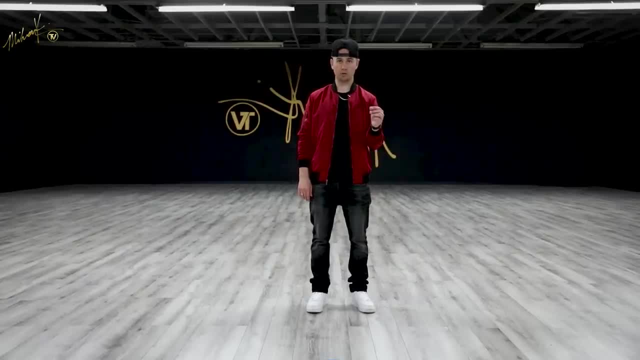 up bam. So that's one, two- We're going to do the same thing with the other arm- Three, four, all right. So we go. five, six, seven, eight. One, two, three, four, all right. 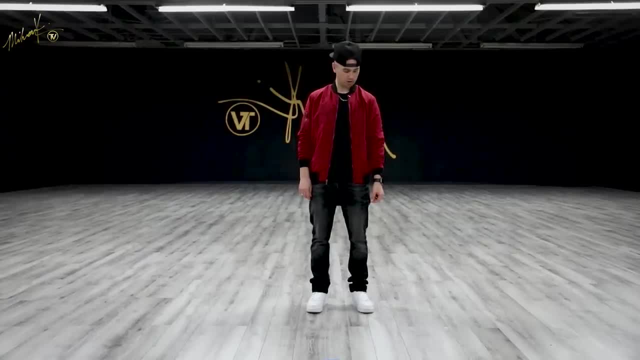 So, each of those positions, I'm going to pivot, I'm going to twist my wrist and then I'm going to bring my arm up and freeze. all right, Twist up, freeze all right. One, two, three, four, Five, six, seven, eight. 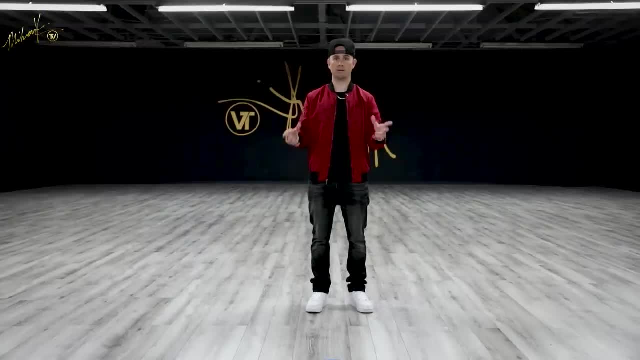 One, two, three, four, all right, Notice that everything else I keep it completely still. One, two, three, four And all those positions. I'm really locking my joints, I'm locking my muscles into those positions, so it can. 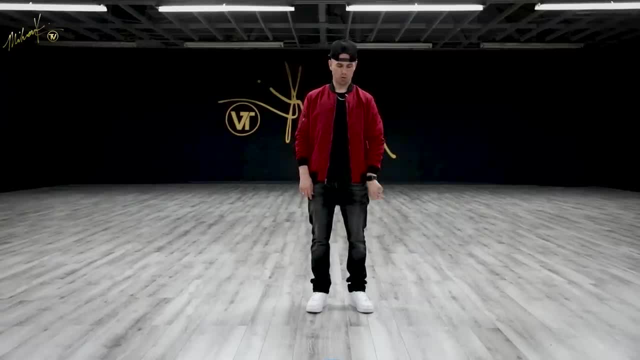 freeze. You don't want to have too much movement. It's going to go. wrist arm- wrist arm. okay, Five, six, seven, eight. Wrist arm- wrist arm. Good, Five, six, seven, eight. Wrist arm- wrist arm- all right. 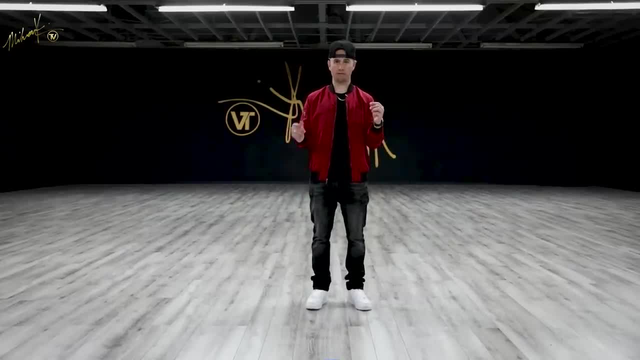 So that's one, two, three, four. Our next move is we're going to tighten up our legs and we're going to pivot to the side. boom like this, all right, So we have our arms up, boom, and we're going to pivot on the heels. okay, So you'll see. 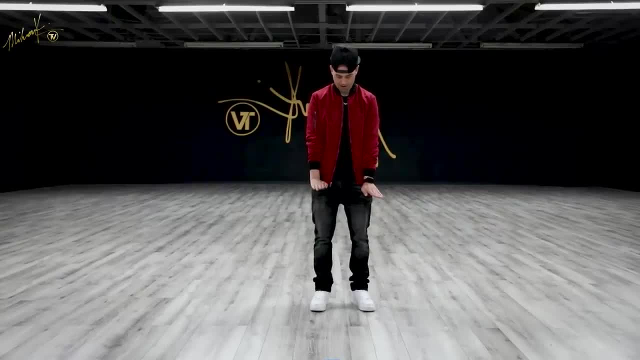 that my two toes, the two fronts of my feet, are going to move together like this, all right. So, basically, I'm tightening up my legs and I'm pivoting to the side on my heels, all right, You don't want to have your feet too high up, all right. So we're going to pivot on the heels, all right. So 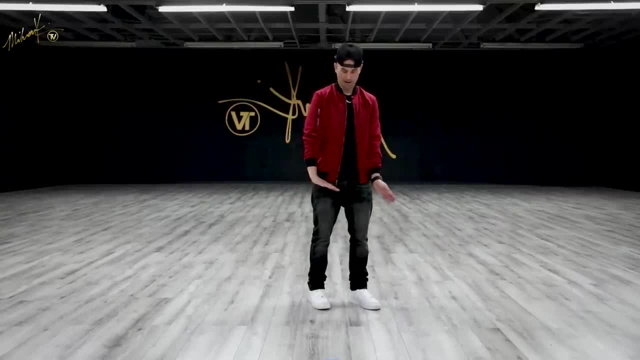 you don't want to have your feet too high up, all right. So you don't want to have your feet too high up, because then it looks like this: So you want them to kind of just skim across the ground: boom, all right. So we're going to go one, two, three, four. we're going to go five, six and we're going to freeze there- all right. So we go one, two, three, four, five, six And you want to stop boom, okay, It really helps if you tighten up your legs while you're doing this pivot, because it makes it really smooth to the side. okay. 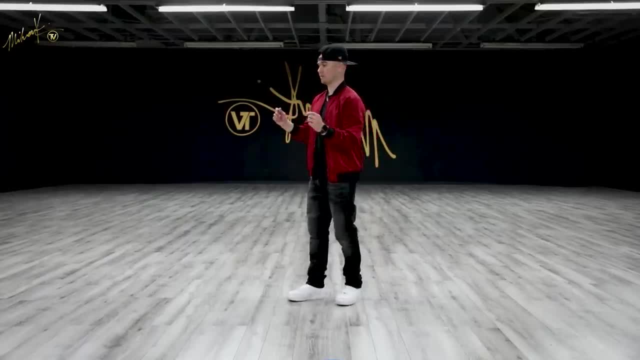 One, two, three, four, five, six, all right. The next move is we're gonna bend down, boom, all right. So that's one, two, three, four, five, six, and we're gonna bend here at the waist: seven, eight, okay. 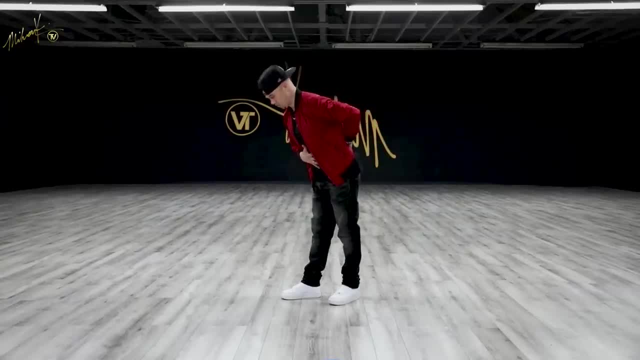 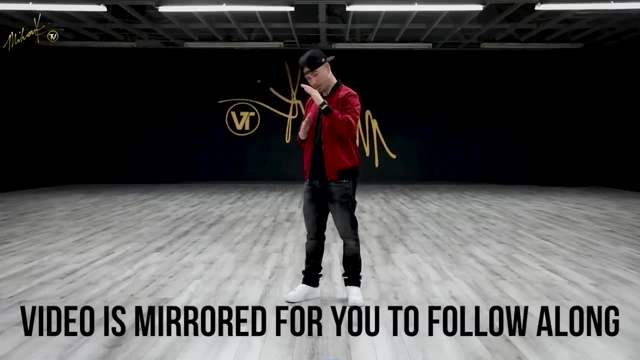 I use my abs and my lower back to really stop that movement. boom, right, You want it to be a full freeze. That's called a dime stop. So I'm moving and I'm stopping. okay, I move, stop, move, stop. 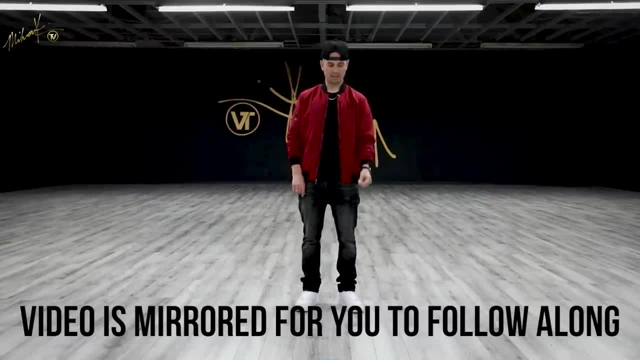 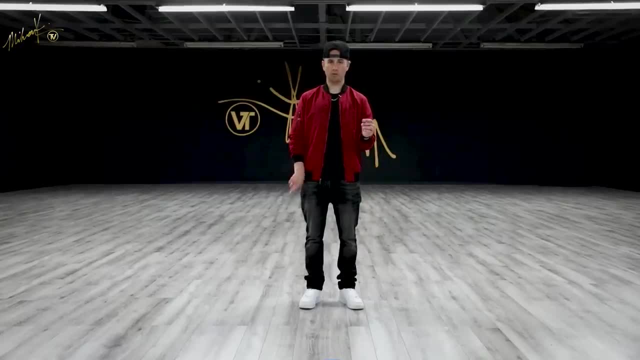 It's really important to learn that dime stop technique in order to get these moves to look robotic. all right, Let's go from the top five, six, seven, eight, one, two, three, four, five, six, seven, eight, all right. 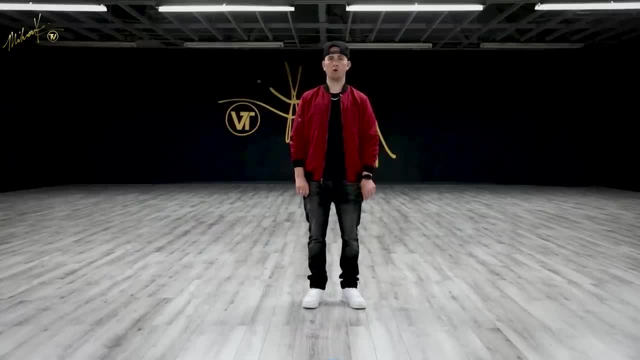 Let's go again: five, six, seven, eight. one, two, three, four, five, six, seven, eight, all right. Let's go again five, six, seven, eight, all right. So I have this pivot boom, seven, eight. 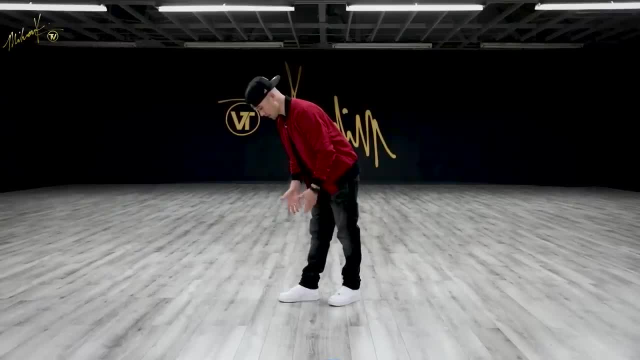 The next move is: I'm gonna bend my knees and I'm gonna bring my torso straight up. It looks like this: It goes boom okay. So I bend my knees and I bring my body straight up like this. So it's almost like this bend that we have in our waist. 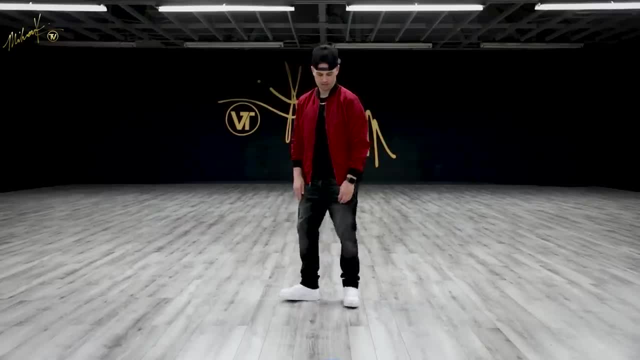 goes into the legs and that bend comes out of the waist. all right, So we have wrist arm, wrist arm, Pivot seven, eight, one, two, We're gonna go three, four, okay, So we have here, and then we're gonna go knees bam. 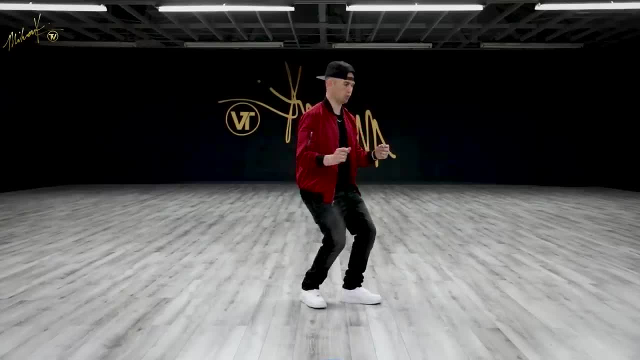 and we're gonna pivot to the other side. So what I'm doing is the same pivot, just in the opposite direction. I'm pivoting on the heels and my toes are gonna go all the way to the other side. all right, But we're in this bent position here with the knees 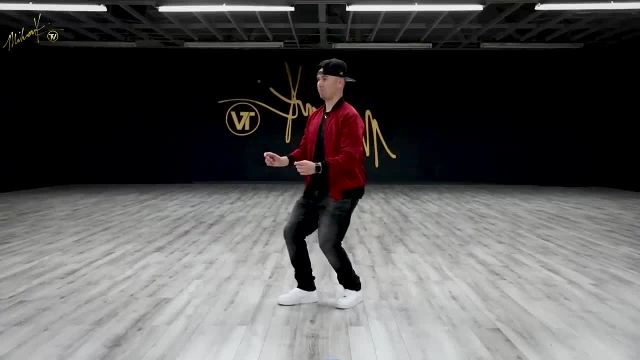 So we're like this: my torso's straight up and down and I pivot to the side. okay, And then the next move is gonna be the legs straightening out. so it's gonna bring us back into that bent position. boom, All right, let's go from there. 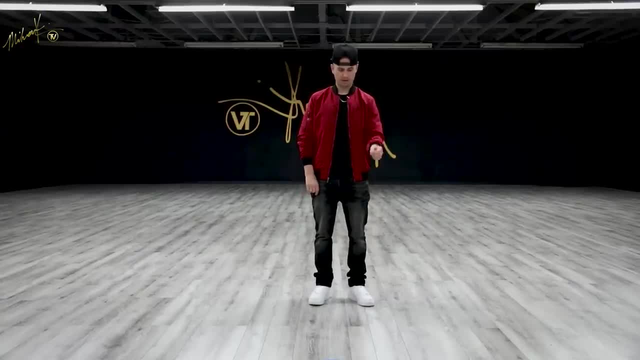 So we got from the top. we have wrist arm, wrist arm, Pivot to the side, Down legs, pivot to the other side legs. all right, So with the counts, it's one, two, three, four, five, six. 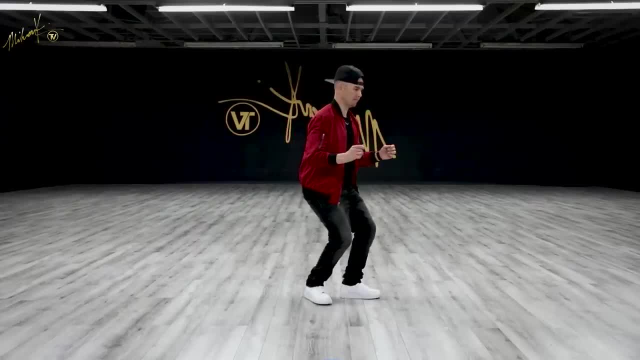 seven, eight, one, two, three, four, five, six. okay, To finish it off, we are gonna bring everything up and we're gonna go here. Basically, what's happening is I'm bringing my arms down to the side. 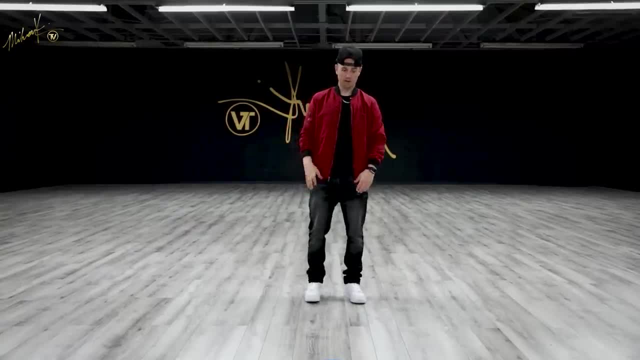 and I'm pivoting at the same time. to be straight forward, The reason we're coming straight forward is we're gonna be able to do this routine over and over again. okay, Since it's two eight counts, we can redo those two eight counts. 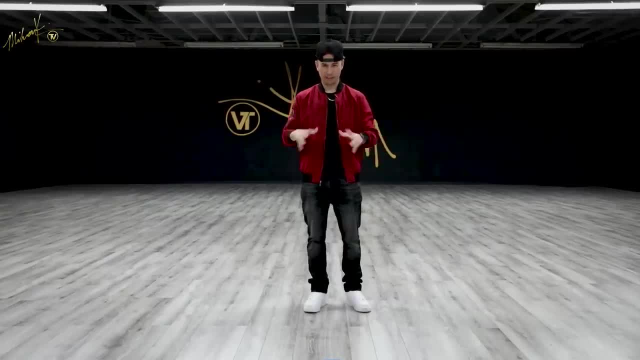 starting from this position. So let's do that a few times slowly, Let's try to get the rhythm down and kind of get those movements, get the pattern down, okay. So here we go. Five, six, seven, eight. 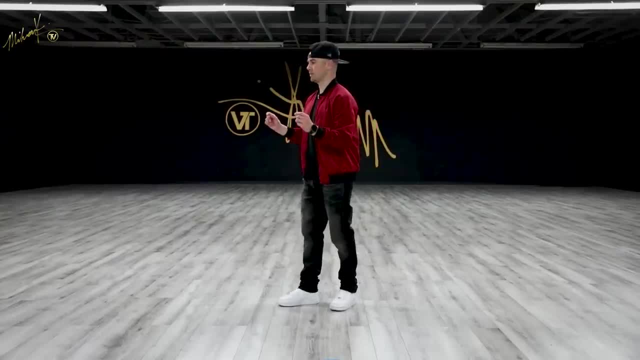 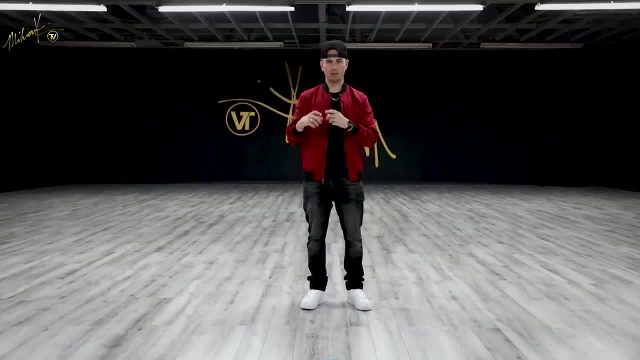 It's really important to really freeze in those positions. Okay, I'm not like just stopping really quick, I'm actually freezing just for a second in that position and then I'm going to the next one, and then I'm going to the next one. You can see that there's pauses in between. Okay, so one, two, three. 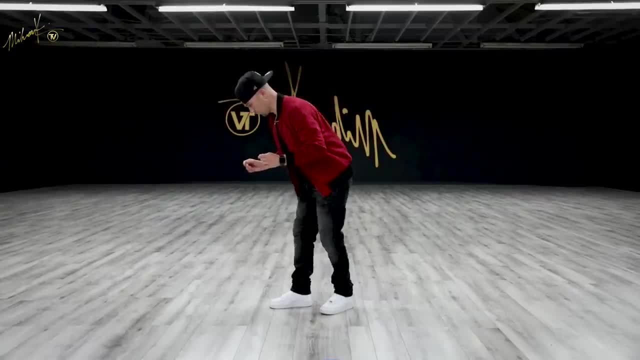 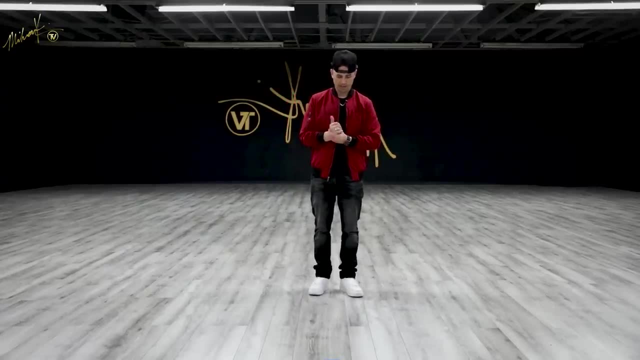 four, five, six, seven, eight, One, two, three, four, five, six, seven, eight. Alright, so that's our two eight counts. Let's go through it kind of like on repeat. We're going to finish here, bam, and we're going to go right into the next one. 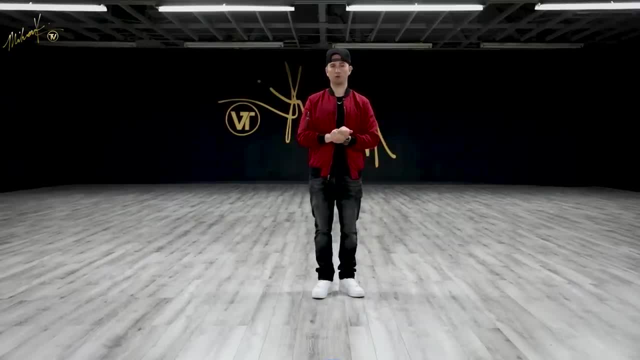 Alright, so let's do it a few times and then we'll do it to some music. Alright, here we go. Five, six, seven, eight, One, two, three, four. five, six, seven, eight, One, two. 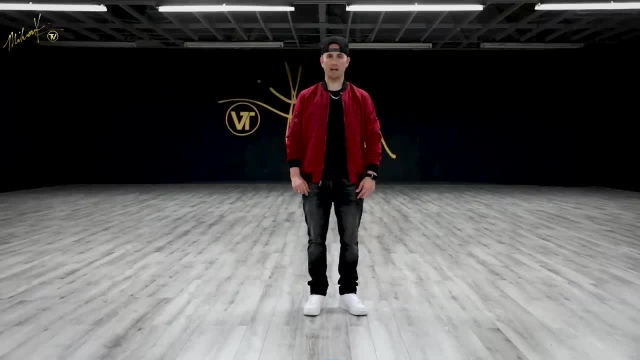 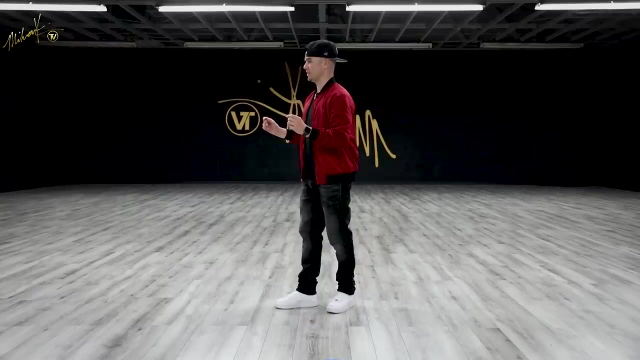 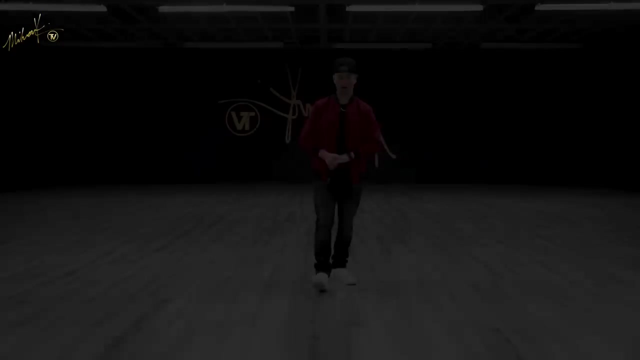 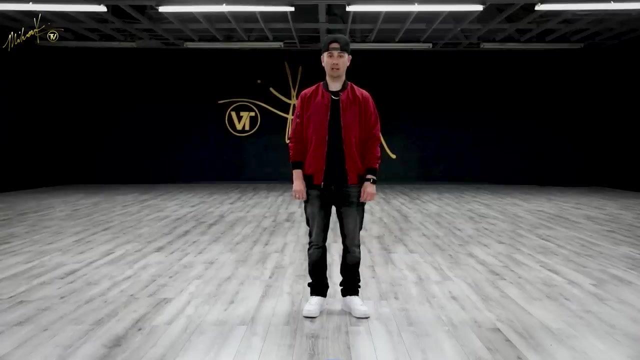 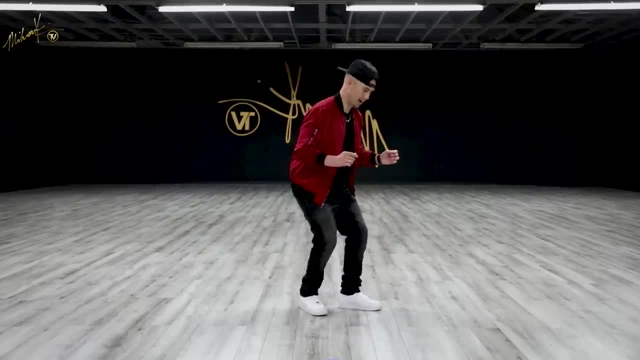 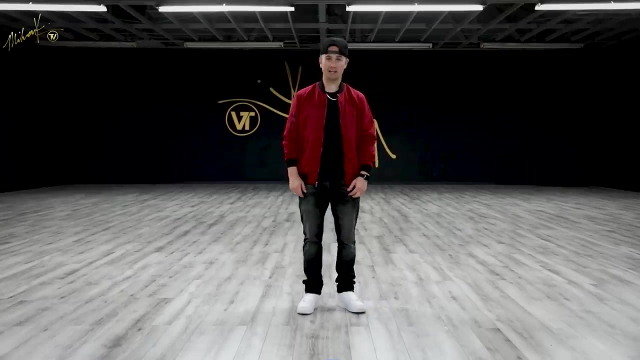 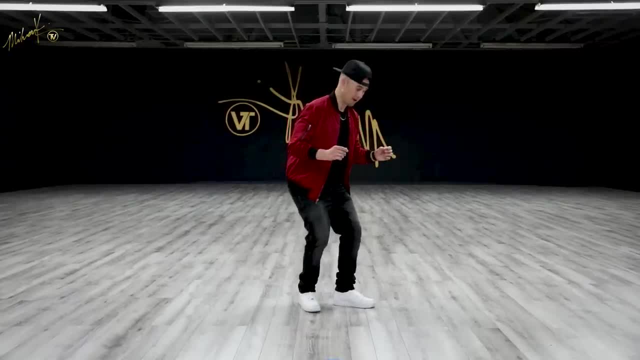 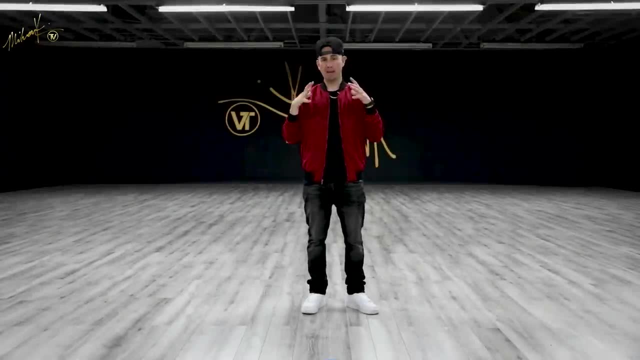 One, two, three, four, five, six, seven, eight, Boom. All right guys, Make sure that you're really focused on all the stops. I'm really freezing in all those positions. I'm really trying to look robotic. 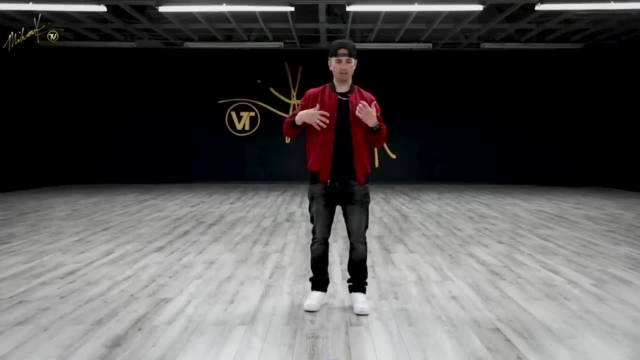 And the other thing is I'm using a lot of energy. okay, It might look like we're just moving and stopping and moving and stopping, But in order to make it look really robotic is I'm using a lot of tension. I'm using a lot of energy. 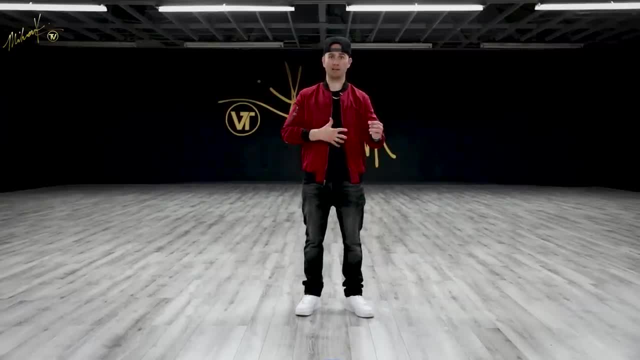 So all of those positions, I'm really flexing everything. I'm flexing my muscles to make it look sharp and robotic, okay, So really focus on all those details And, again, you need to repeat all of these positions, all of these moves. 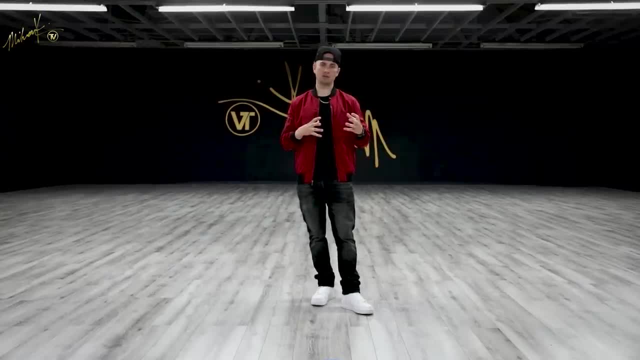 Really get the transitions down And then you can start to, you know, apply more energy into it. You can like spike, You can spice it up with different flavor And yeah, it's all about the journey Practice. 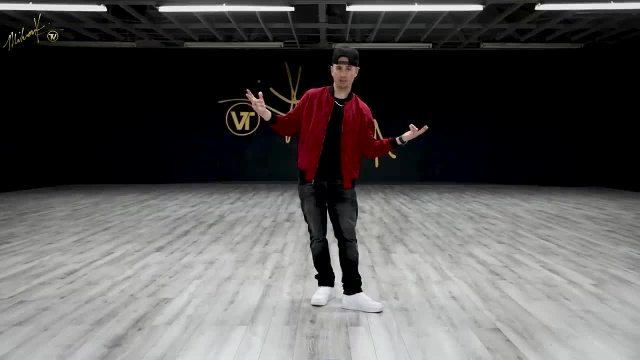 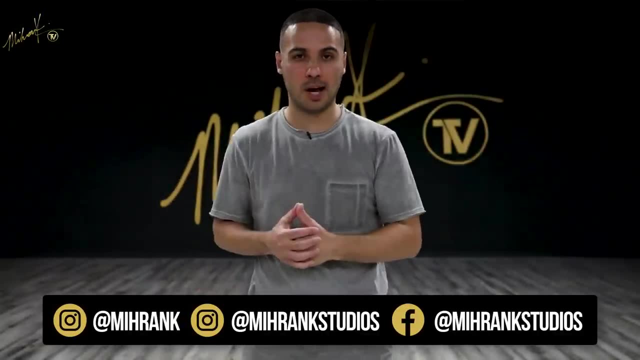 Really get these positions down And on to the next one. All right, guys, Poppin' John here. Peace. Hey guys, I hope you enjoyed this tutorial with Poppin' John. If you're still having a hard time with the basic robot dance, watch the video again. 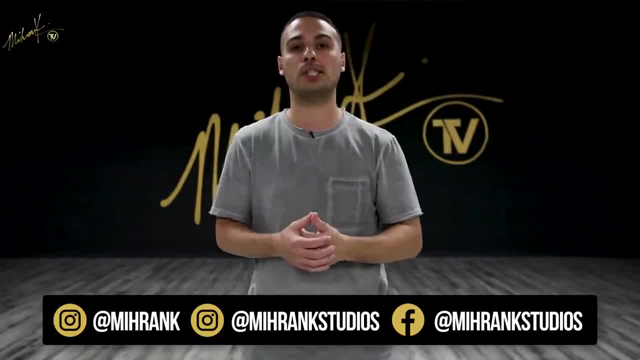 Review all the details until you feel confident. If you want to know more information about Poppin' John, I will put all of his links in the description box. Also, if this is your first time watching, please subscribe to my channel. 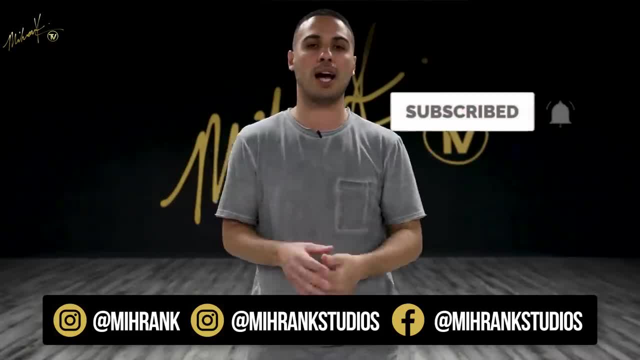 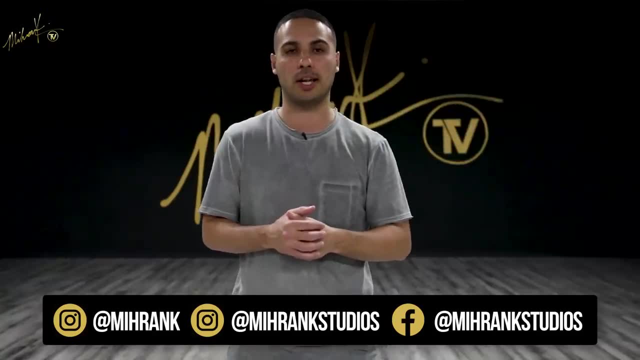